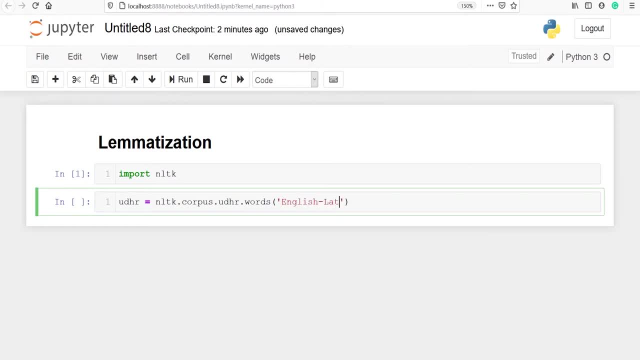 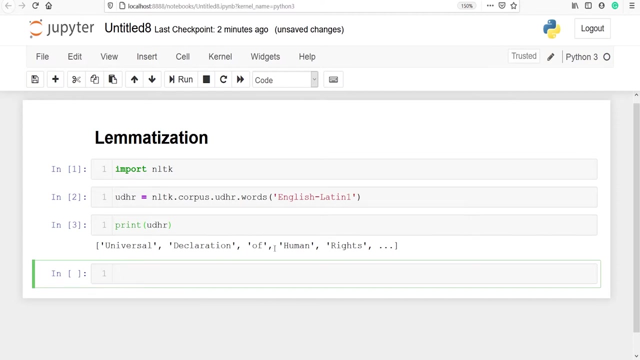 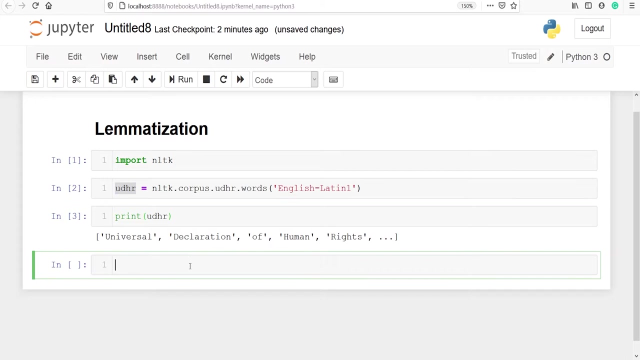 English. Let's execute our code. Let's print our variable UDHR. We have some words like universal declaration of human rights. To look at more words, we will use UDHR. Then we want to look at, let's say: 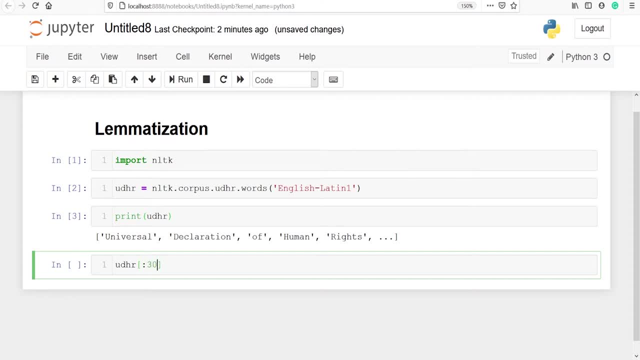 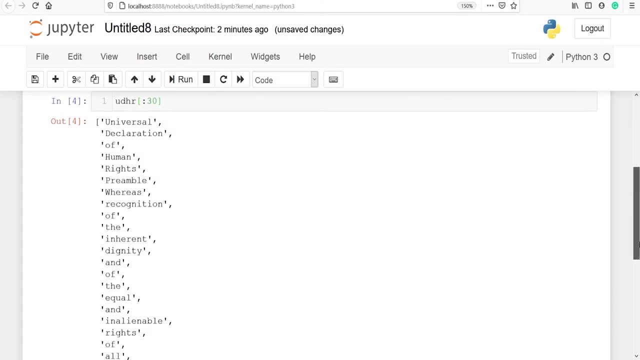 first 30. words. Let's execute our code. In the output you can see that these are the first 30 words that are present in UDHR and the words are: universal declaration of human rights, preamble, etc. First we will apply stemming. I will make one variable voter and from NLTK I will call. 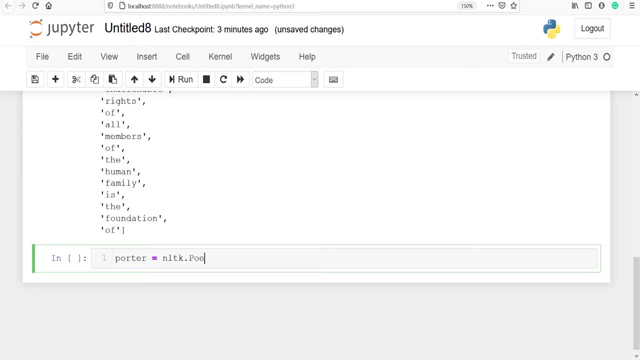 the class. This is the method. Let's say, for example, the word stemmer. let's write the class. We will use UDHR here. have a few words and I will also create a list Here. we will call the class. 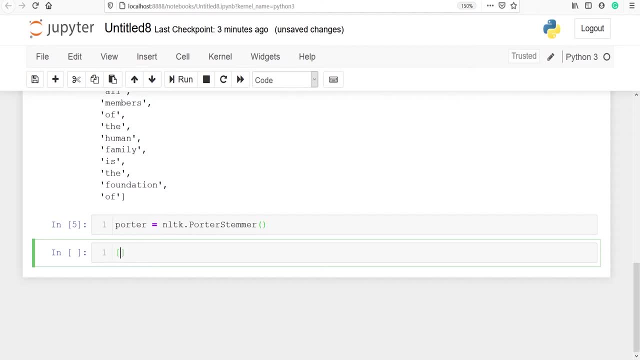 Now we are ready to execute the code. Let's execute the code. Let's write the string. Let's say, for example, the word stemmer From the string, I will write the space- UDHR may be the space- and in the output you can see that we have a word stemmer. Let's write the. 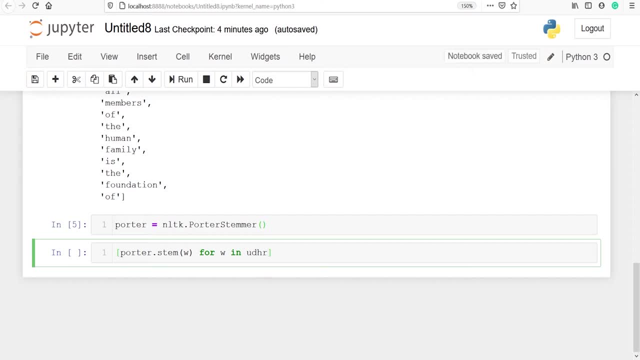 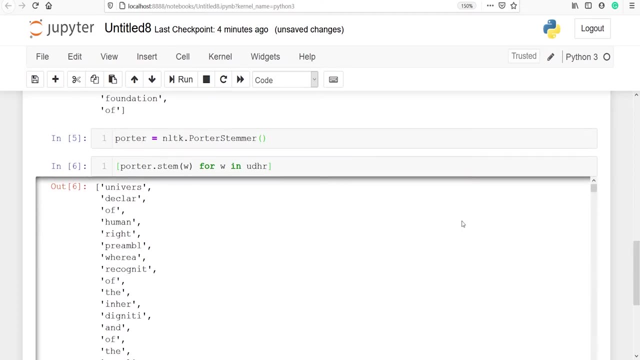 message. The code gets entered in a string. I will make a list comprehension. I will call our object porter. Let's execute our code From Porter. we will call the method. stemmer have applied stemming and you will see the result here. universe declare of human rights. 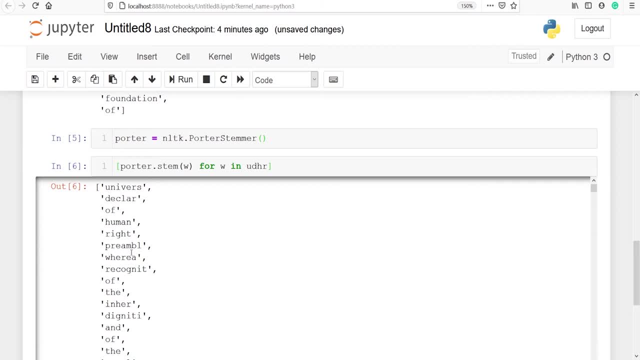 you will see, words have been trimmed and they have become meaningless, such as universe, declare, preamble, recognize and so on. now these are. these have become meaningless because these words are not meaningful. and here comes lemmatization. lemmatization would do stemming, but keep the. 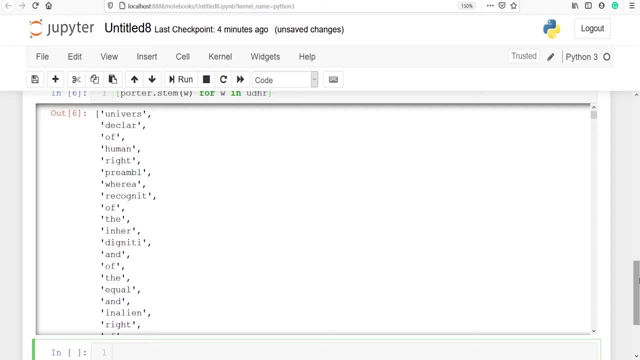 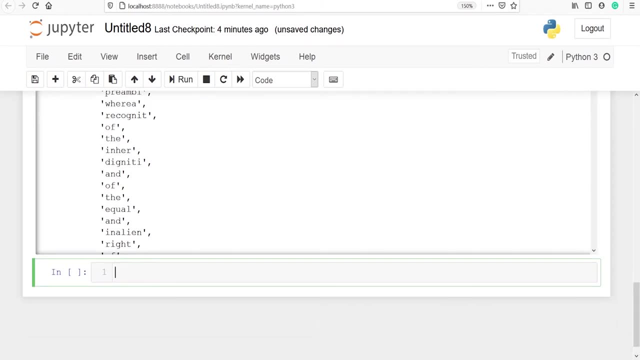 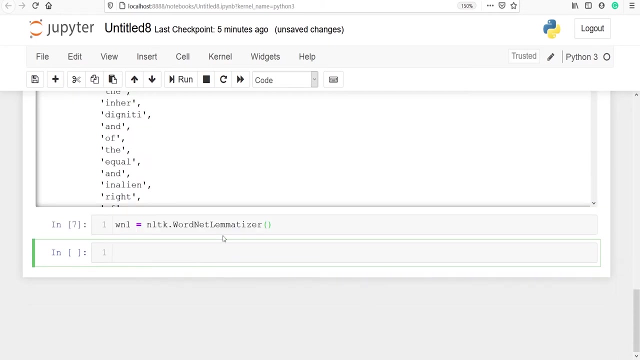 resulting tense to be valid words. we will use the method word net lemmatization. from nltk i'll make one variable, wnl, and from nltk i will call word net lemmatizer. let's execute our code. we have saved this class in this object, wnl. now i'll make a list comprehension. 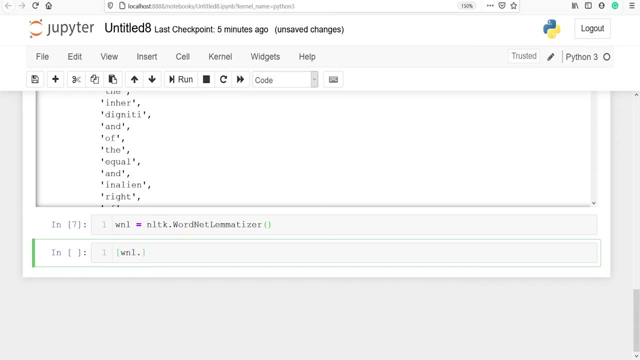 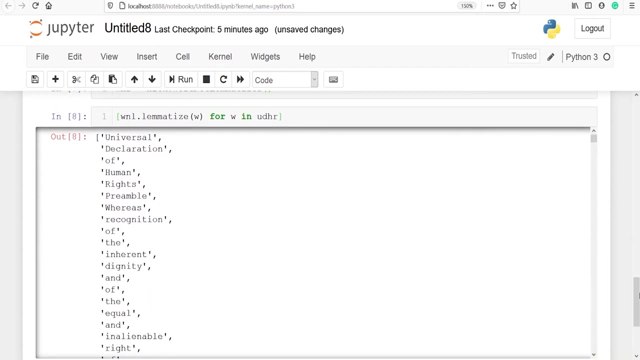 from wnl our object. let's call the method lemmatize and then we will write a loop w for w in udhr. let's execute our code in the output. you can see that we got the result here and we have done lemmatization. 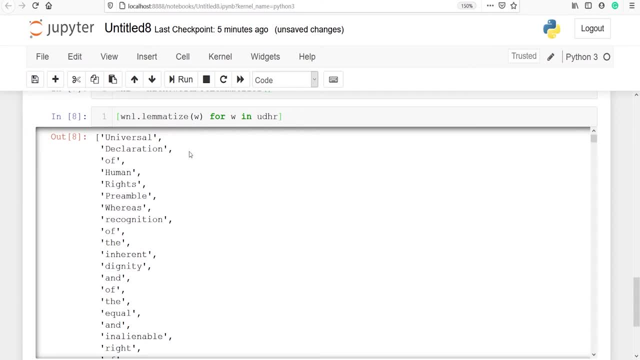 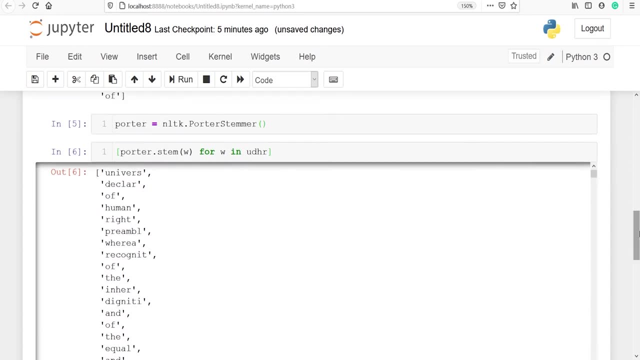 and the words are meaningful. universal declaration of human rights preamble. whereas. but if you look at the above method, stemming, the words become meaningless. here, universe is not a meaningful word. declare is also not a meaningful word. so in some cases we have to apply lemmatization so that we can keep. 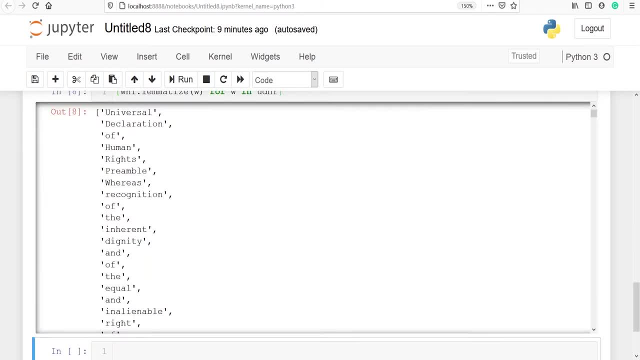 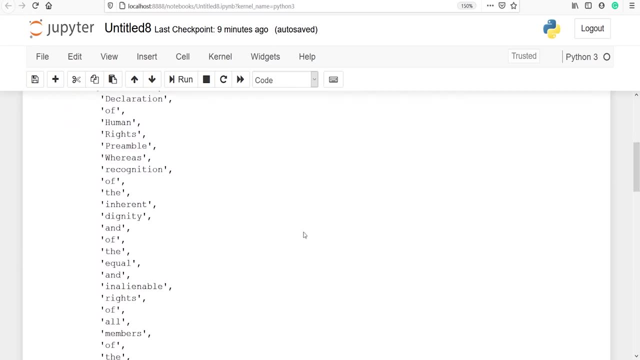 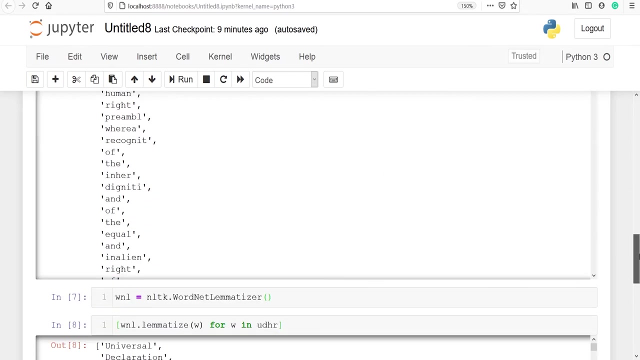 the word as meaningful. how do we know that lemmatizer has worked? if you look at the original, you will see here. you will observe that after inalienable, we have rights and rights has s here. and if you look at the current result after lemmatization, you will see that, after inalienable, 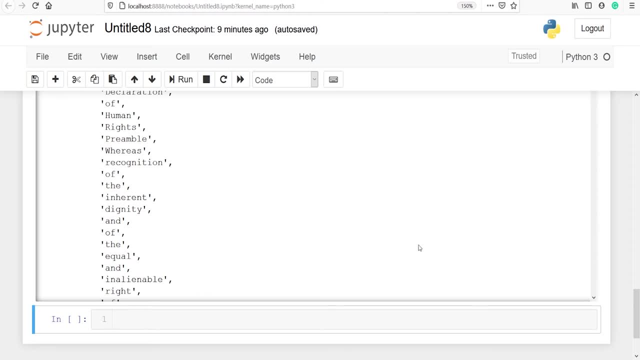 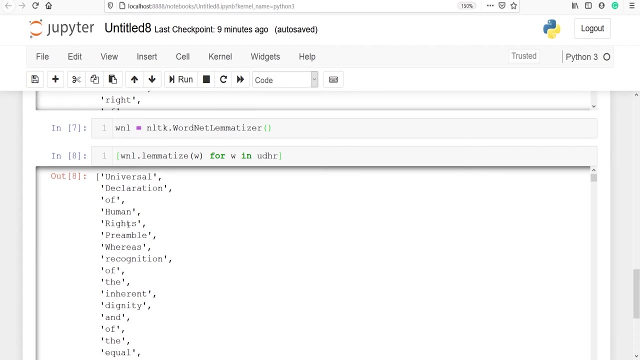 we have right and the s has been removed. that means lemmatizer has been performed on this, and here you will see we have human rights and here also we have s with rights and in the original variable you have mental right and here you will see, we have s with right and the original variable. 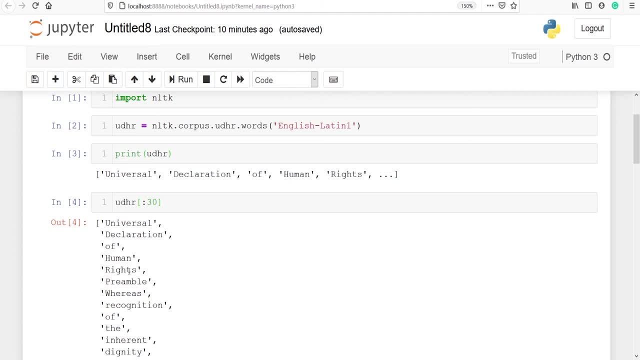 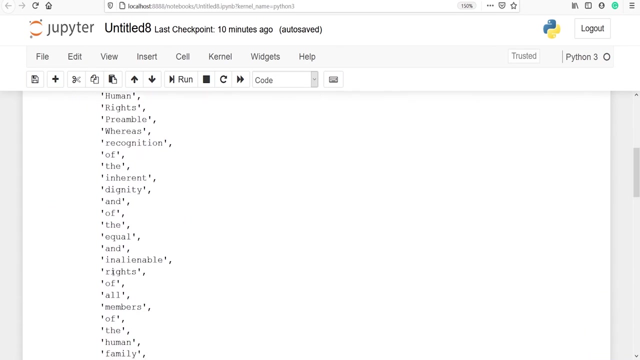 in the original UDHR. here also we have rights. the reason is because this rights is in capital letter, the R is in capital letter and that is why the S has not been removed from this right. but here in rights, this rights is in small letter, the R is in small letter. that